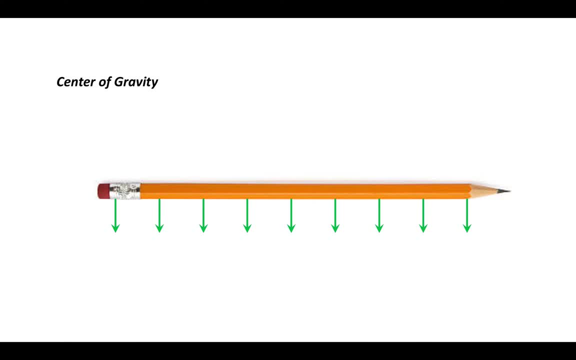 those small scales would register a little bit of weight, because the weight of a pencil is distributed fairly evenly. That can be represented as a center of gravity. If you imagine balancing a pencil on your finger, all of that can be represented the sum of each one of those. 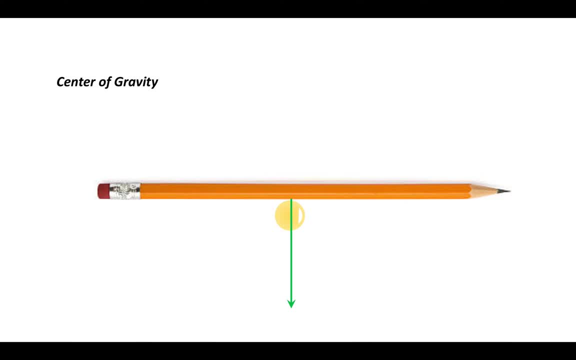 little scales as a center of gravity. So let's talk about center of gravity. Now let's talk about center of buoyancy. So now let's imagine we drop our pencil in some water. The water is pushing up on the pencil and it does this because the pencil floats. Why does? 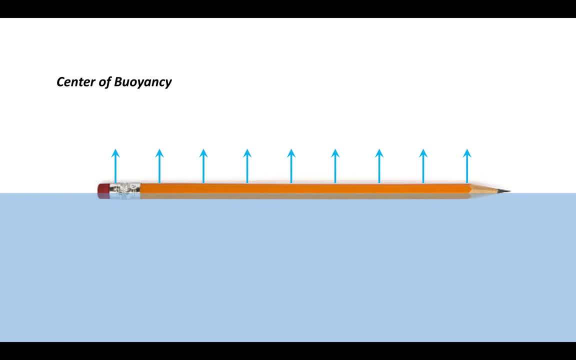 the pencil float Because the surface area of the pencil displaces an amount of water that weighs less than the pencil, and so, therefore, the pencil floats. Just about any material can float. It all depends on how much water it displaces and what the weight of the material is. 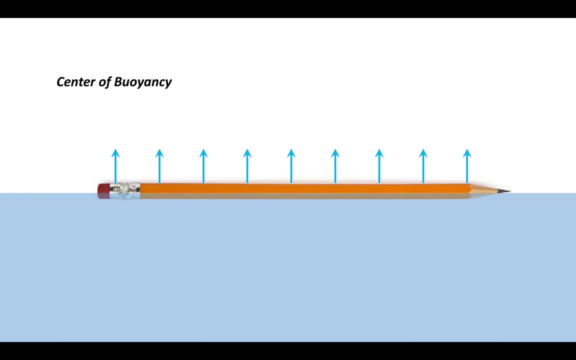 And so, just like the center of gravity can be represented around a single point, this one's a little harder to imagine, but if you can imagine, like balancing a pencil on the tip of your finger, pushing up, if you could balance it on the tip, that could represent the center of buoyancy. So 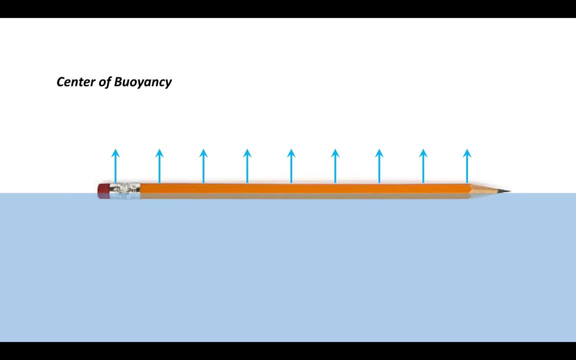 just like you could balance a pencil on the tip of your finger, you could balance it on the tip of your finger. you could take all of the sums of those arrows to represent the center of gravity. Same thing: center of buoyancy. So we have those two concepts If you think about all of the points. 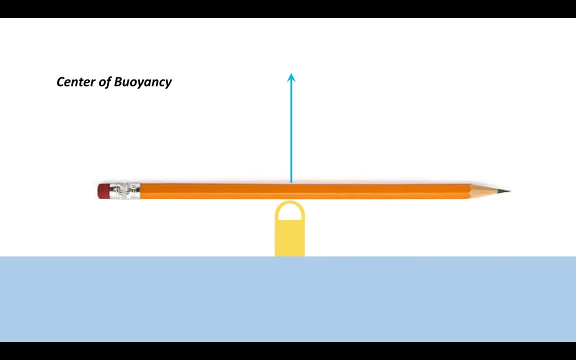 of where something weighs and all the points of where something makes it float being concentrated in one point, And from a physics perspective, that's the way you model things. So now let's take a boat. So imagine this is any boat looking from a stern. So imagine this is like Serenity. 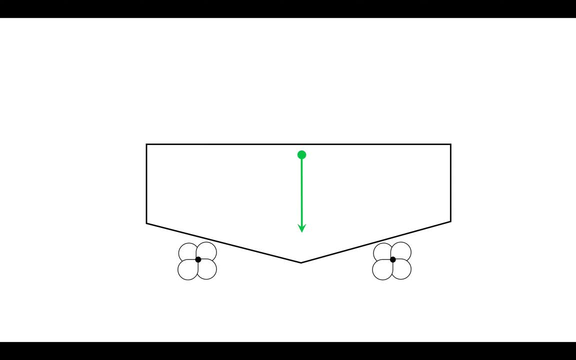 as you're looking At the stern of Serenity. So Serenity weighs some amount and there is a center of gravity. If you had a really strong finger, you could, in theory, balance Serenity on one single point, And that. 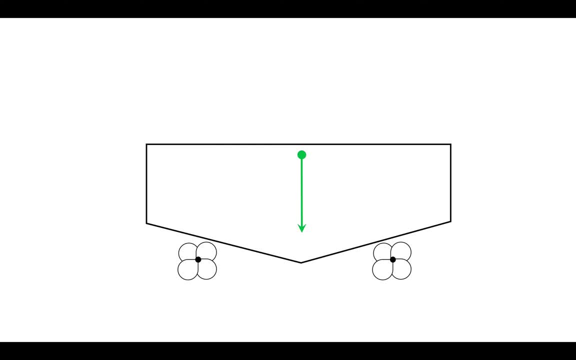 would be the center of gravity. The sum of all of the weight across all of the boat, both side to side in Florida could be measured in one single point. Here we're really worried about boats- tipping is what we're talking about. So we're worried about that center of gravity left to 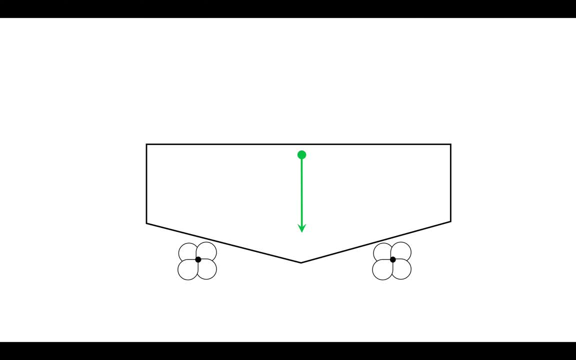 right port to starboard athwart ship, however you want to refer to it. So the side to side center of gravity. So there's some point that's directly on center line and then, based on how much the boat weighs at the bottom versus middle versus the top, there's some representation of the center of 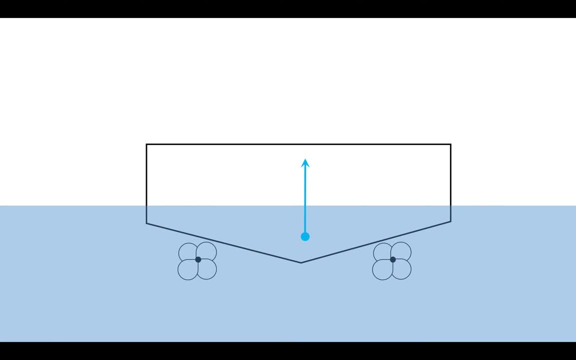 gravity. Similarly, when you put a boat like Serenity in the water, all of the water that gets displaced, however much, whatever the weight of the water that gets displaced, is what the displacement of a boat or the weight of a boat is, And that can be all represented in one point. 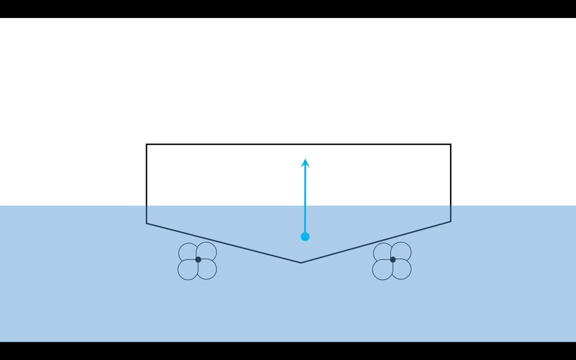 that is someplace below the waterline. So it's a representation of the force that the water is exerting to make the boat float, all concentrated in one point. Here again, left to right is the. we're thinking about this. So when you put those two things together, there is a center of gravity. 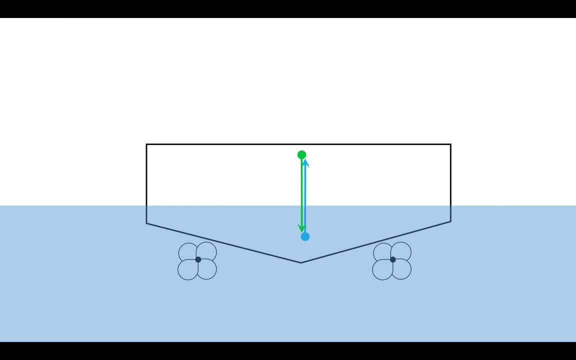 pushing down, That's the weight. There's a center of buoyancy. pushing up, That is the water pushing against the boat that keeps it afloat. So a boat at rest with nobody on it, nothing moving around, no wind blowing on it, that's what it's going to. 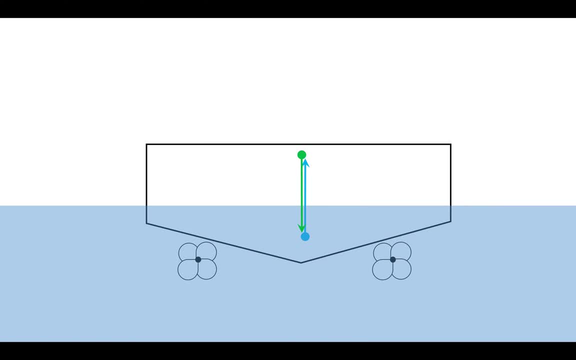 look like It's going to be stable and it's going to sit there and float, which is the natural state for not only boats, but anything that floats in the water. So now let's talk about what happens if someone was to move around on the boat. So let's say you had some people. step to the right. 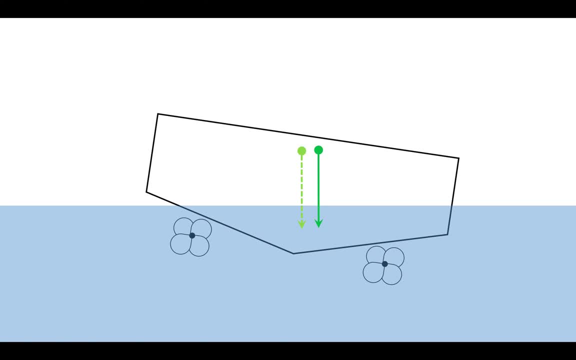 side of a boat. Well, what's going to happen to this person? Well, they're going to have to center of gravity. If the people move to the right side, the center of gravity is going to move to the right side and the boat is going to tip to the right. Now, those people relative to the boat, 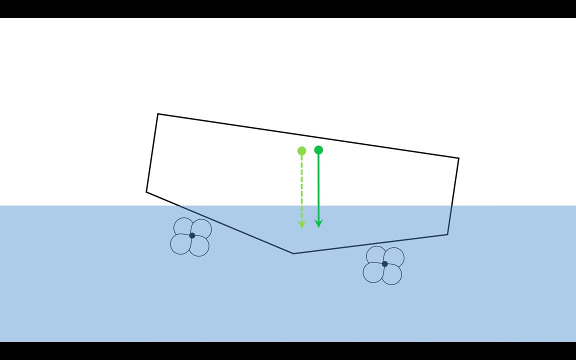 don't weigh very much. If you imagine a paddleboard, if you were standing in the center of a paddleboard and you took just a little step off to the side all of a sudden, that's going to have a big impact. But on a boat that weighs a lot, taking a small step is really not going to have much of. 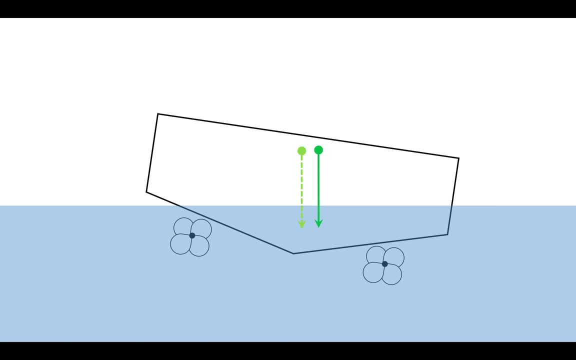 an impact on the shift of the center of gravity. But something else interesting happens as well: When the boat tips a little bit, the center of buoyancy also moves right. So, and this is why boat bottoms are designed like they are, because with this little 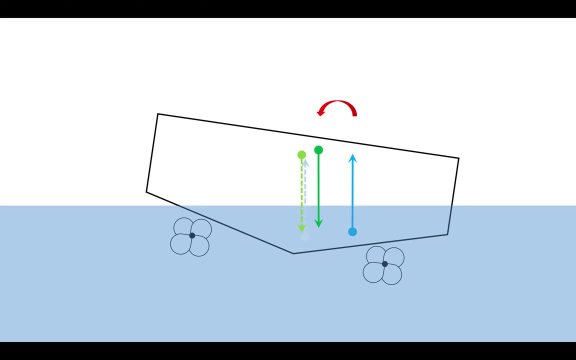 bit of a V-cut, it's technically called a dead rise. When that goes down in the water, the center of buoyancy actually shifts well to the outside, Because again you have to imagine that the sum of all of the area, if you could find the center of the area, of the part of the hull- 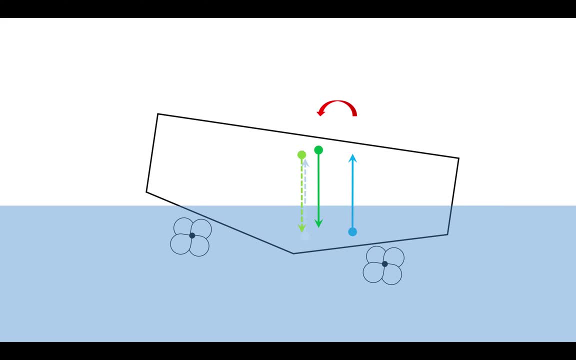 that is underneath the water that's going to represent the center of buoyancy pushing up, And so boats are designed, almost by nature, to have the center of buoyancy shift further and faster than the center of gravity does, which basically creates a torque effect. So if you 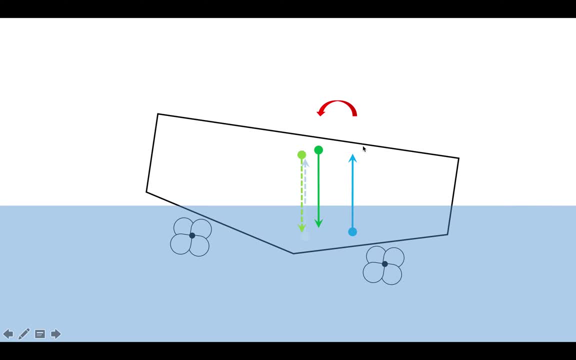 could imagine the blue arrow pushing up. so this arrow is pushing up and this arrow is pushing down. What does that want to do? It wants to turn the boat rack back towards a normal state, To where the center of gravity and the center of buoyancy are basically offsetting each other. directly opposing each other, which will keep the boat stable. So boats are designed. the shape of the hulls are designed to be able to promote that. If you had something that was flat, like a paddleboard, for example, that center of buoyancy doesn't shift as much, which is why a 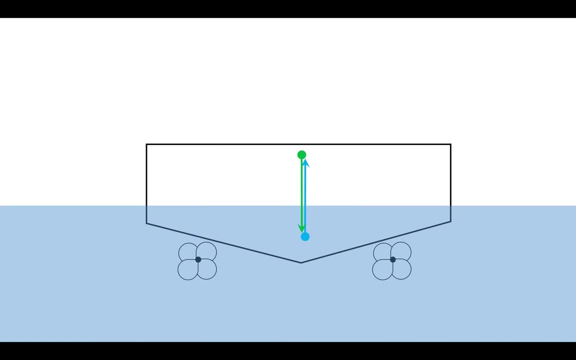 paddleboard is so unstable. As soon as you get weight on one foot on the side of a paddleboard, you know there's not an additional amount of water that's being displaced because the bottom of the board is flat and therefore that's why paddleboards like flip-flops. 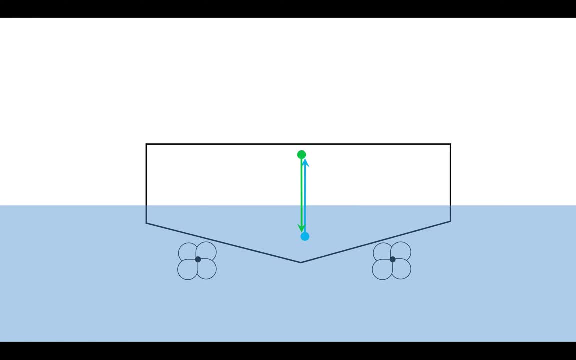 so easily. But boats are very different because they have this V-cut, and we'll talk even a little bit more about the concept of ballast. So I know one of the things that I think you were concerned about was the accident that had happened on the 4th of July back in 2012,, which was a terrible. 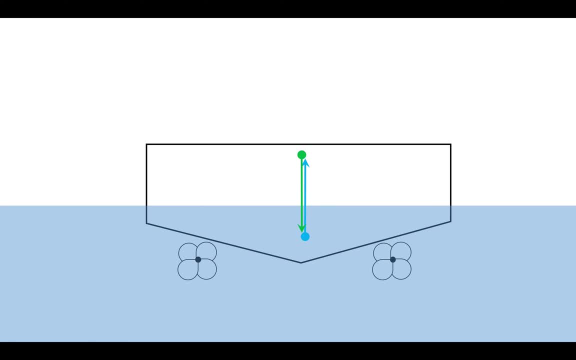 terrible situation, obviously, But you know, I read the accident report and have read it multiple times. I read it when it came out and I reread it again And let's explain what happened to that boat. So imagine we're looking at the stern of that boat. So that boat was a 34-foot. 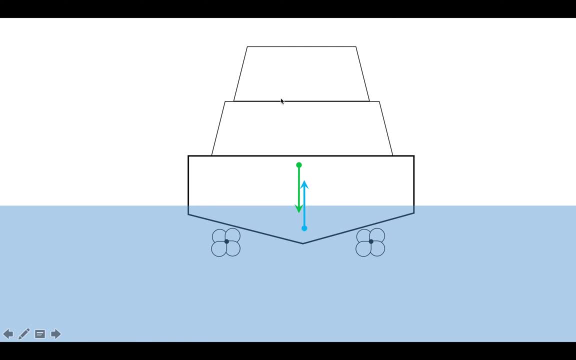 Silverton that had a you know cabin. So this would be, you know, much like our boat, like Serrani, but it also has this flybridge up here on the top. So the investigation found that the weight of the boat was 16,500 pounds empty. So once they got the boat out of the water, 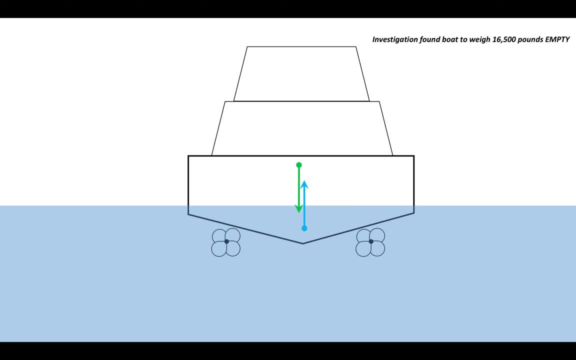 first of all, they knew the make and the model of the boat, but the specific boat- they did testing on it- They determined that that boat, empty, would be 16,500 pounds- is how much that would weigh. And these are important numbers so you can understand. 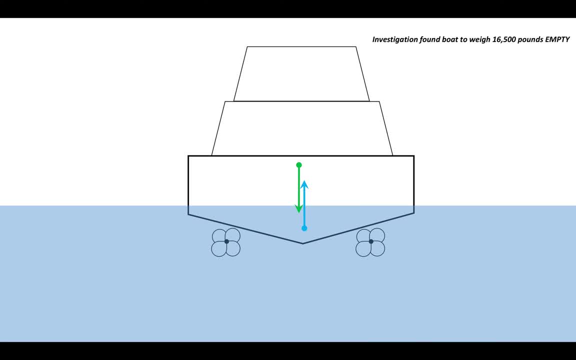 you know kind of the relative nature of this. There's some complex math that goes behind this where we could explain the riding moment based on angles. I mean it gets into fluid mechanics. We're not going to do that, So this is intended to be a simple analysis. 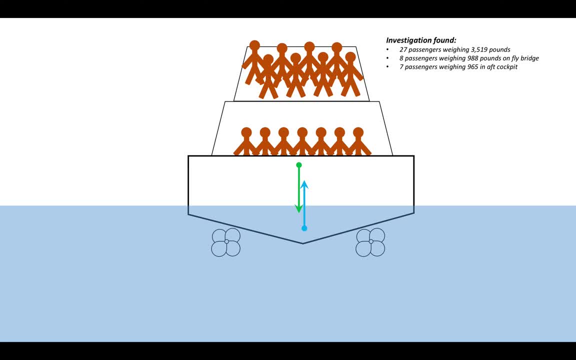 Here's what else the investigation found. The investigation found that that boat had 27 passengers on it And those 27 passengers were on board. So that boat had 27 passengers on it, So that's 27 passengers. in total weighed 3,519 pounds. It was an average of about 130 pounds per. 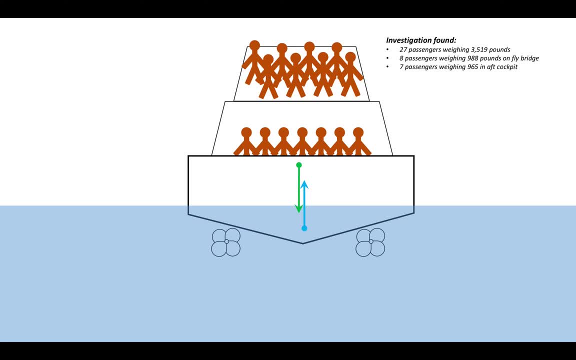 passenger, There were some older folks, There was some adults. you know number of kids ranging in ages On the flybridge. so up on top, which would be catamount to standing on the roof of Serenity, there were eight passengers which weighed 988 pounds on the flybridge And there were seven. 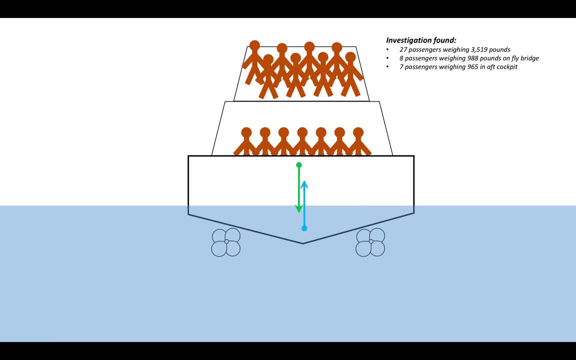 passengers in the aft deck that weighed 965 pounds, The passengers then inside five total that were in the cabin and the remainder were actually up on the bow. So this boat was like it was crowded because it's a 34-foot boat. So here's what. 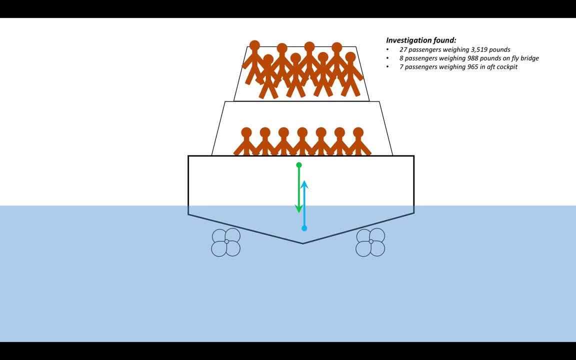 happened that night leaving Oyster Bay. The investigation found that there was a lot of boats that were leaving. He was running at about half speed somewhere in the 12 to 15 knot range in boats because there was a thunderstorm coming and I think boats were trying to get by quickly. 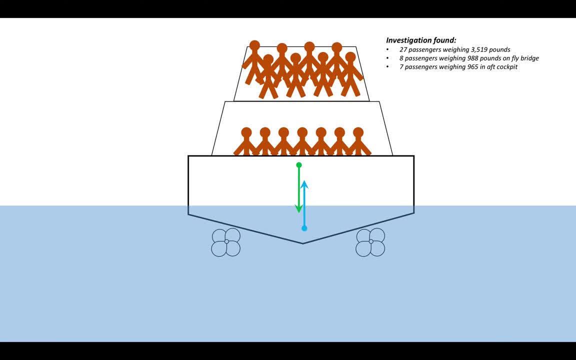 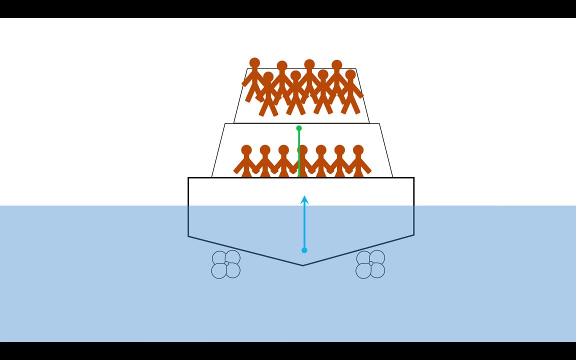 And so boats had been going by left and right, And so the first thing that happened is, because of all those people, the center of gravity is much higher. right, Because people are up on the flybridge, the center of gravity raises and the 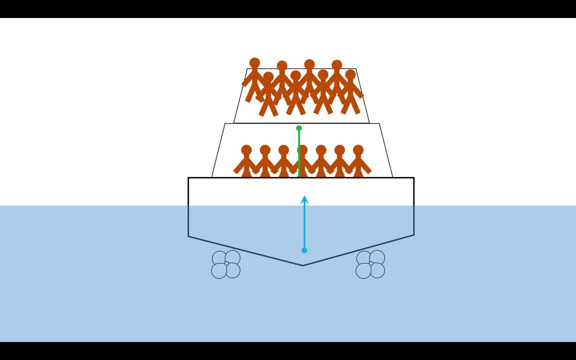 center of buoyancy lowers because it also caused the boat to sit lower on its lines. Whenever you put weight on a boat, it's going to set a little bit lower on its lines. So that was the first thing that happened. The second thing that happened- and this, by the way, makes the boat 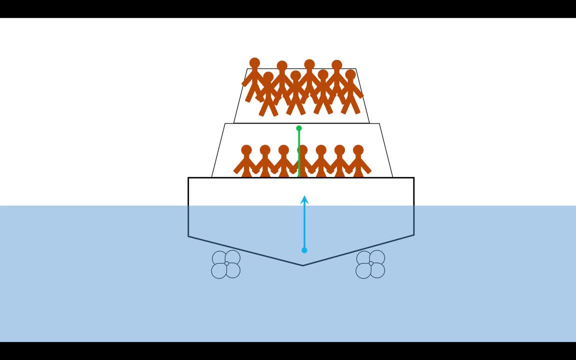 naturally less stable because, in theory, having the center of gravity and center of buoyancy almost at the exact same point would be the most stable kind of boat you could have. which cruise ships are designed to be that way, And we'll talk about that at the end, so we can talk about the cruise. 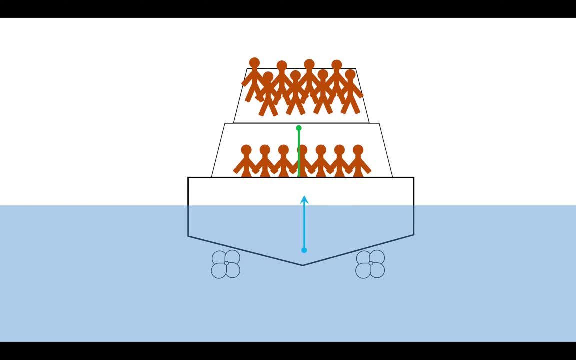 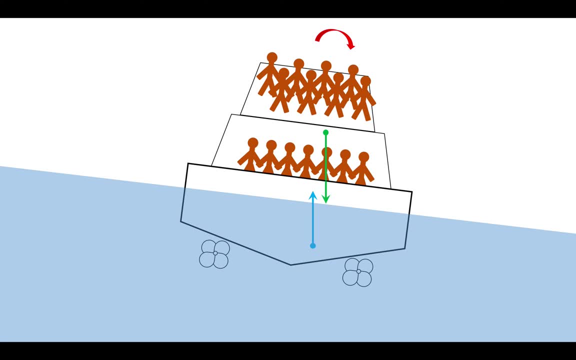 ship example. But this separated the center of gravity and the center of buoyancy, So with all these boats going by, that created some waves. The accident found that, given the way the boat was loaded, that it would have only required a two-foot wave. 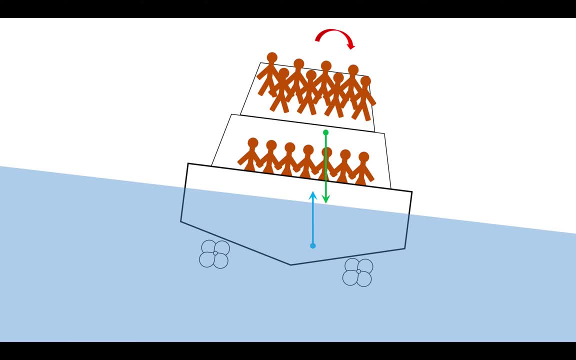 To get the boat to an unstable situation which would have caused it to capsize. We see two-foot waves all the time. I've had serenity abeam in 15-foot waves. I mean, being in a situation where a boat could capsize in two-foot waves is crazy, which is why there was just so many people on. 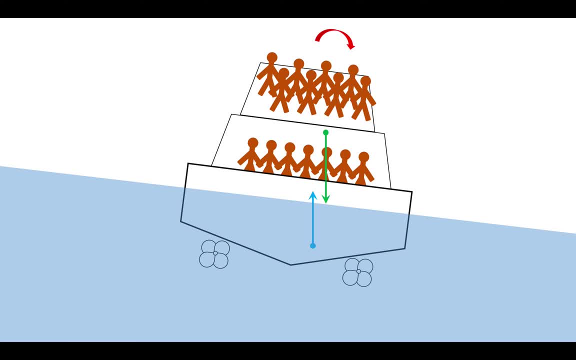 this. So basically what happened? right, because it was sitting lower on its lines, the center of gravity didn't move. sorry, the center of buoyancy didn't move as much when this uh started to tip. So this represents kind of a subtle little wave here. but the center of 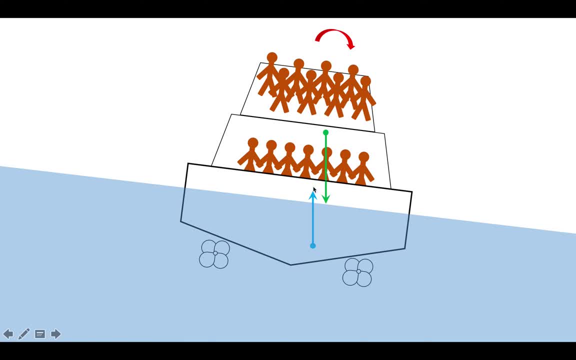 gravity shifted out to the right. And as soon as this center of gravity, the green arrow, as soon as it got on the outside of the center of buoyancy, you start to have trouble, Because now, if you can imagine the pressures working on the boat, this is pushing up. this is pushing down, which makes the 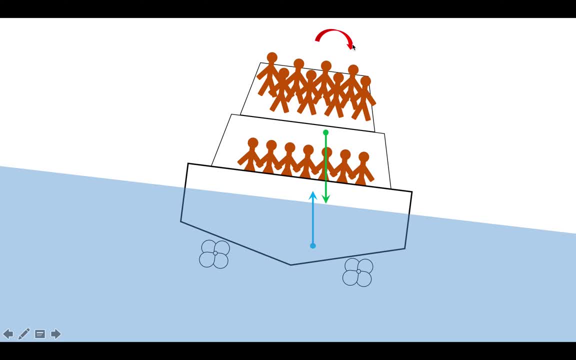 boat want to turn even further And they talked about how they could feel the boat starting to tip And and, of course, when the boat leans, that actually makes the boat want to turn to the left, because you just, the way you know, physics, work with something down here which makes the boat. 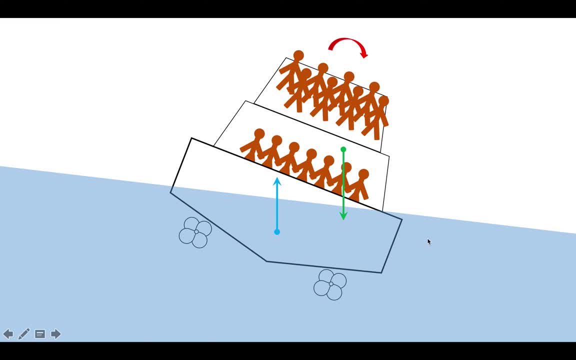 want to tip even more to the right And then you get in the situation where, once it tips just enough, you started to get water coming over the gunnel, uh, over the rail, which they talked about. uh, in multiple, the witnesses talked about how they can start to see the water coming over the rail. 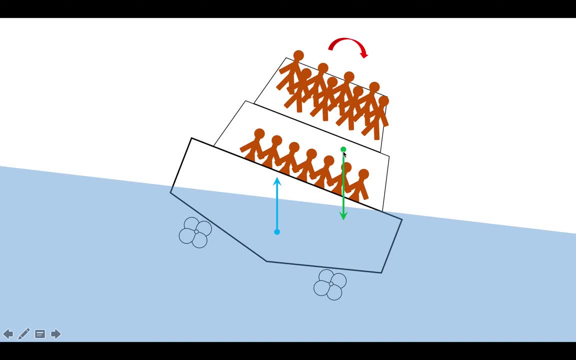 of the boat, And what that is going to do is shift the center of gravity even further out and the center of buoyancy is still going to remain about the same. And at this point, uh, fait accompli, I mean it was done, The the boat was going to capsize and it happened very 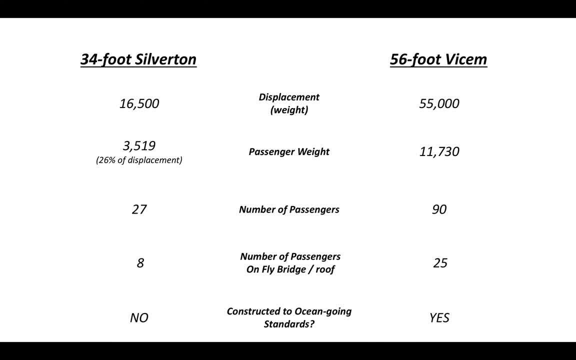 very quickly. So let me talk about a reference point here. right, So that was a 34 foot Silverton. We have a 56 foot feature. A displacement on that boat was found to be 16,500 pounds. Our boat displaces 55,000 pounds, So a lot more, almost four times as much. 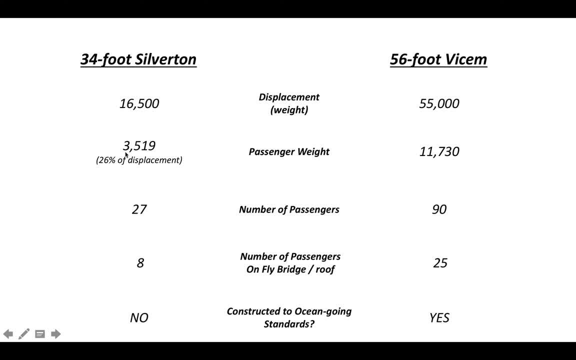 Their passenger weight was found to be 26% of their displacement: 3,519 pounds, That's 26% of the 16,500.. For us to have 26% of our displacement on Serenity, we would need 11,730 pounds. So on. 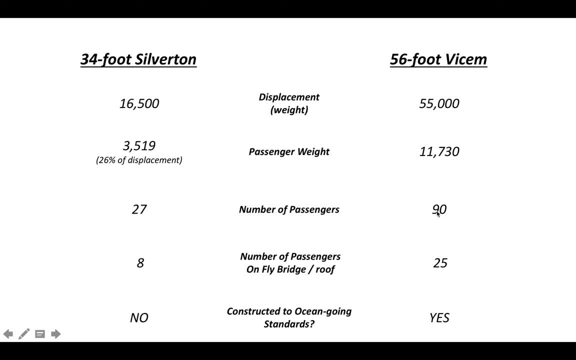 the 34 foot Silverton that was 27 people. On our boat it would be 90. So them having 27 people would be the equivalent of us putting 90 people at the same average weight of 130 pounds onto our boat. They had eight passengers on their fly bridge, again on a percentage of 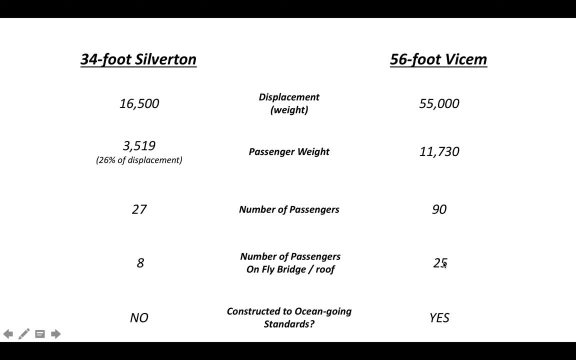 of weight displacement. That would be like us putting 25 people up on top of our roof Um with, by the way, 90 people total. So so so 65 people on the rest of the boat and 25 people on. 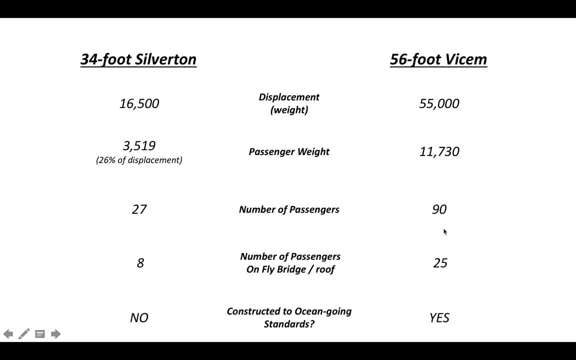 the roof. you know, not just 25 people on the roof, So it'd be 20, it'd be 90 people on the boat with 25 on the roof would create a similar condition to what this 34 foot Silverton is in. 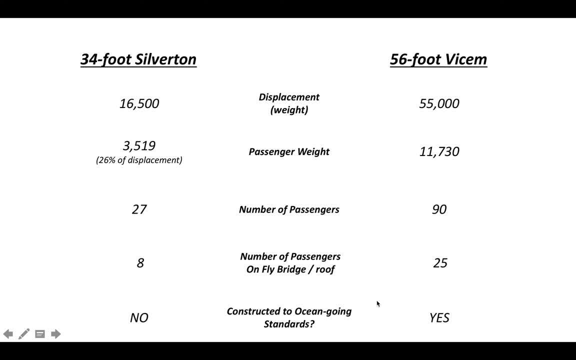 Um, and then actually it would even be as bad, because one thing about our boat is our boat is constructed to ocean going standards, And I won't go into the details here. Uh, but there are are two councils in the world who basically set forth guidelines for boats that are going to. 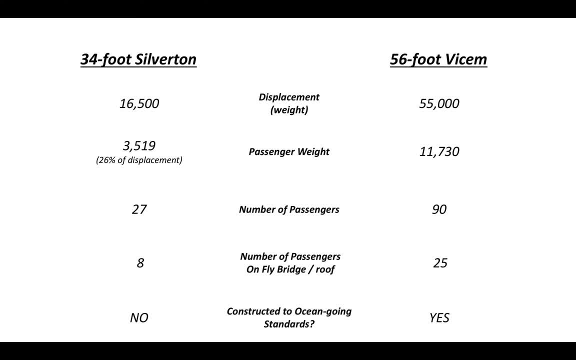 operate on the high seas, And our boat is designed to that, Whereas the 34 foot Silverton is not. it's designed to be a coastal cruiser, And so it actually does not meet either one of the requirements, Uh, and, and one of those requirements is a greater riding moment. So 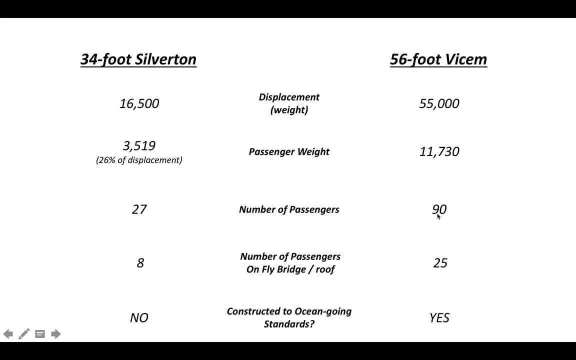 even if you did have this situation, if you had 90 people on Serenity and you had 25 of those people standing on top of the roof and we were going at 15 knots and a two foot wave hit us a beam And you know I turned the wrong. 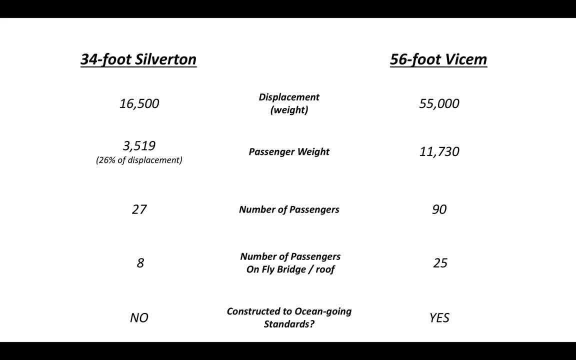 way on that. I still don't think our boat would capsize because I think it has a much greater level of stability than the 34 foot Silverton. So that is why boats in general, and, you know, our boat in particular, are so safe. This was a very bad decision. 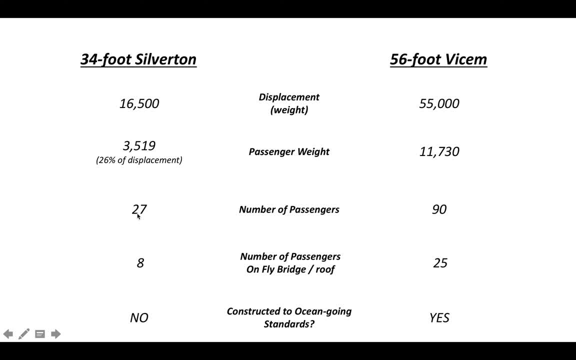 on the part of the captain. Uh, I get it, It was 4th of July. They thought they were gonna go out on calm seas and have a, have a enjoyable night, but but you should never, ever have this number. 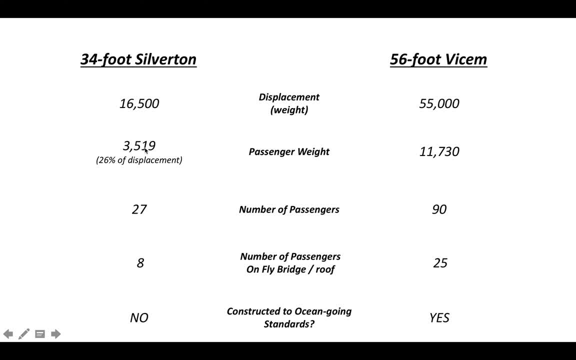 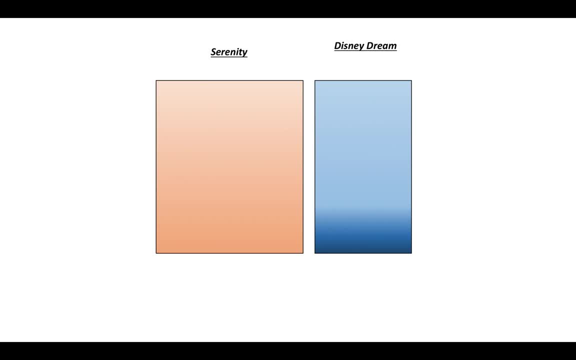 of people on a boat. um, that creates this kind of uh ratio of passenger weight to displacement. So we'll talk about one more thing. I want to talk a little bit about our trip on the Disney dream, And and. so what I want to show you here is: this is our boat and this is the Disney dream. 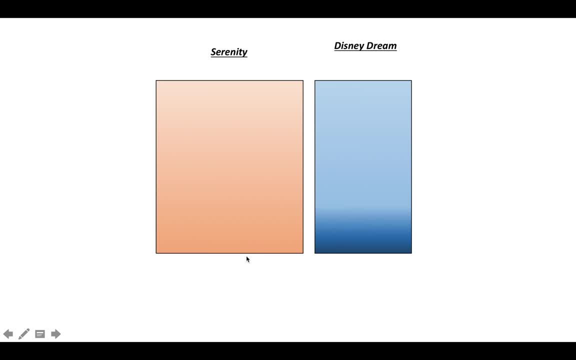 and this is for the total height of the boat, So from the top of the boat all the way down to the bottom of the keel. So, um, you know, serenity and is, and, and I'll show you the numbers. but if you 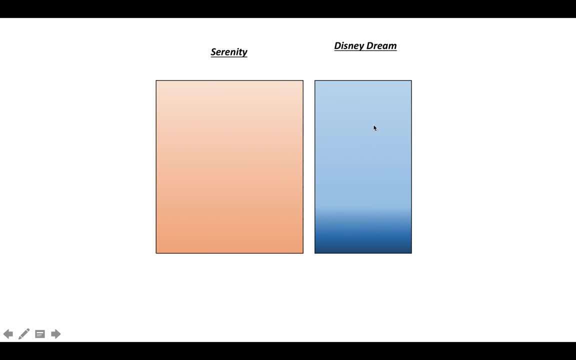 imagine these two things being, you know, scaled so that they were equal height. you can tell that the Disney dream is a narrower, narrower boat. I also did this color scheming because, you know, the weight is really concentrated at the bottom of the Disney dream. So let's overlay these. so 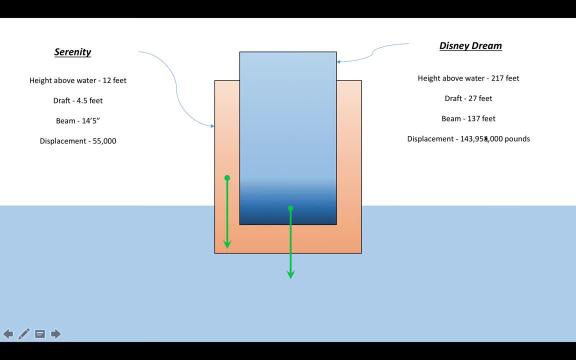 you can get a feeling for what these look like. So if, if you were to go out on a boat and you're on a boat and you were to overlay these and again so that they're the exact same height, even though obviously they're not, they're vastly different ships. but this just helps understand. 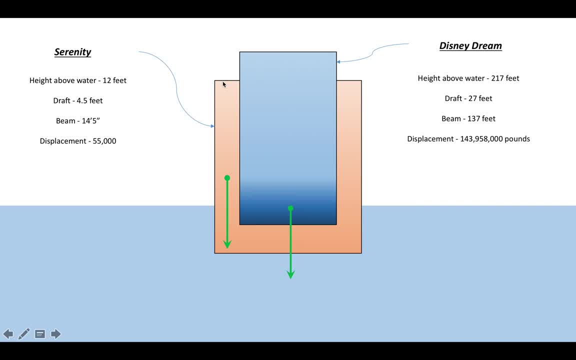 So. so here's the numbers on serenity. So serenity is about 16 and a half feet total from top to bottom. 12 of that is above the water line. Four and a half is below the water line. Uh, the beam is 14 and a half feet and we displaced 55,000 pounds. And so this green arrow to the 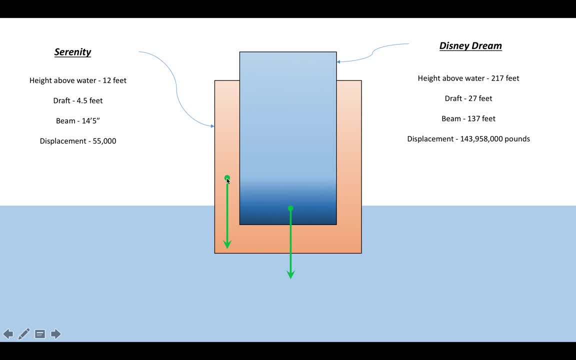 left- that's in this, you know kind of orangish color represents our center gravity is is above the water line. uh, for sure. Uh, I mean our, our boat would tip over if it was turned 85 degrees on its side, but it's never gonna happen. Uh, it would be almost. 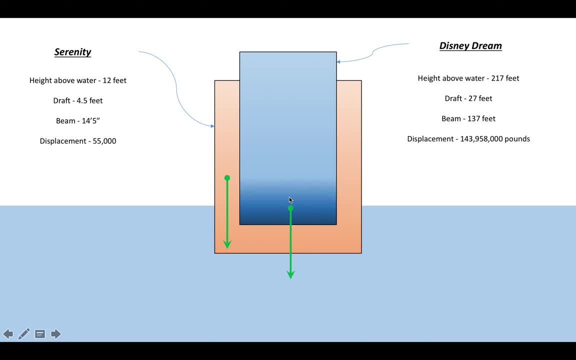 impossible to tip our boat over. Um, but the Disney dream, because not only is the the construction material heavier and all of the engines are below the water line, but they've also got this huge, uh steel bulb that runs the length of the boat. 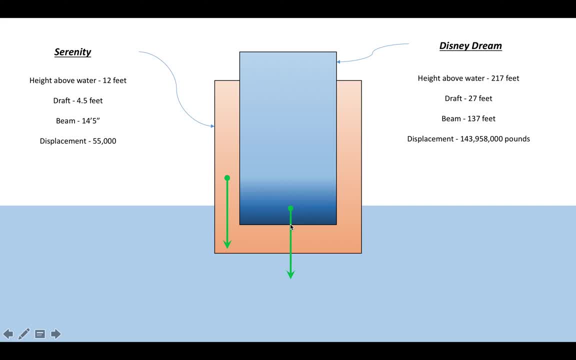 And probably almost half of the boat is- is in that weight of that keel, of that big bulb that runs down the center. So, even though it sticks up more out of the water, uh, on both an absolute and relative basis, and it's narrower, uh, the center of gravity on that cruise ship is actually. 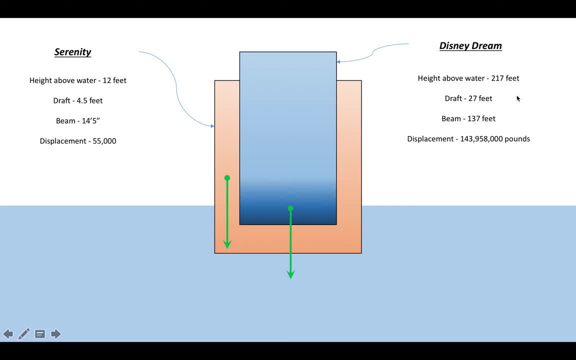 lower. And just so you know the numbers, the height of the Disney dream above the water is 217 feet. It's draft is 27 feet. Uh, it has a beam of 137 feet and it displaces. are you ready for? this 143. million 958,000 pounds. 143 million 958,000 pounds, That is a huge amount of weight. So that's what it displaces when it's, you know, in in. you know it's completed mode without people. 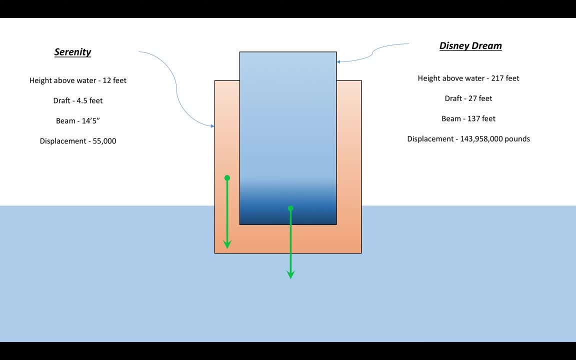 on it. And so the next thing: people look at these big cruise ships and they're like, oh my God, there's so many people going on it, How could, how could that possibly not cause the boat to tip over? Well, check this out on a relative basis. 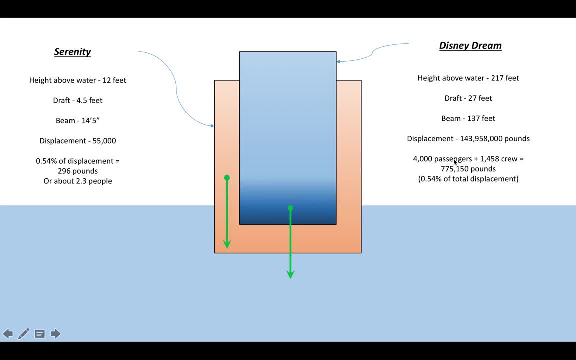 So the Disney dream has the ability to hold 4,000 passengers and, uh, about 1,458 crew. So if you make some assumptions about the 4,000 passengers being about the same weight as the 27 people that were on, uh, the 34 foot Silverton and the crew being all adults so much heavier, that equates to 775,000 pounds. That's how much the total totality of the people would be If you had basically 5,500 people get on the Disney dream. that is 0.54% of the total displacement- 0.54.. I want to go. 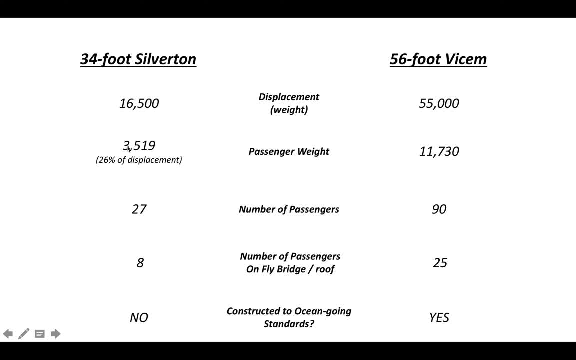 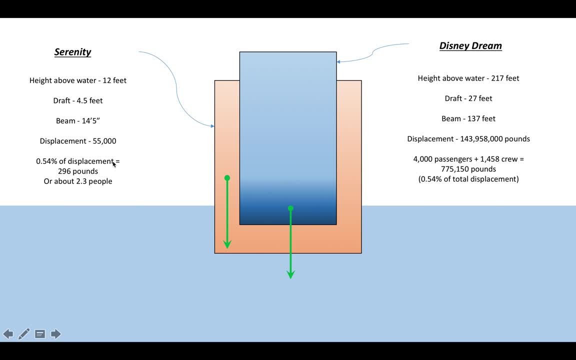 back and show the number again And one more time here: that 34 foot Silverton had 3,519 pounds. in those 27 people, 26% of the displacement. You fully load up the Disney dream: 0.54, not even. 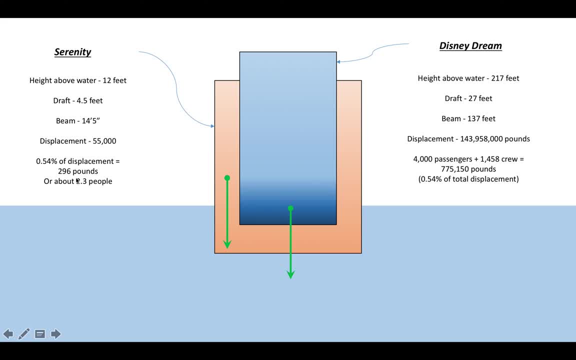 1% of the total displacement comes on. That would be like putting 296 pounds or 2.3 people at an average of 130 pounds. This is like you know. this is. you know, uncle Joe and I get on. 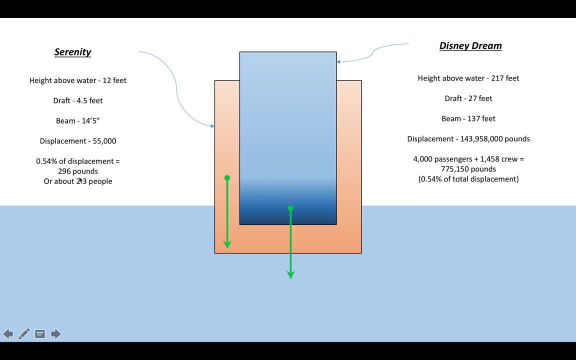 the boat. You and I get on the boat and, and, and and. it's this much. So you know, just like on Serenity, you could put 300 pounds on a rail and the boat almost doesn't even tip. You could have. 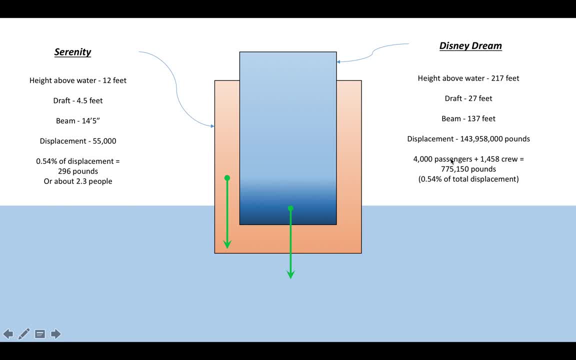 all 5,500 people on the Disney dream walk to one side of the boat on the highest deck and the boat wouldn't even feel it because there's so much weight down low, It just wouldn't even matter. Uh, and so that's why, even though I know it was scary-